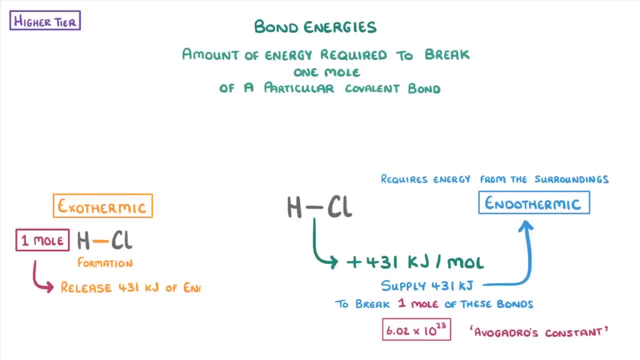 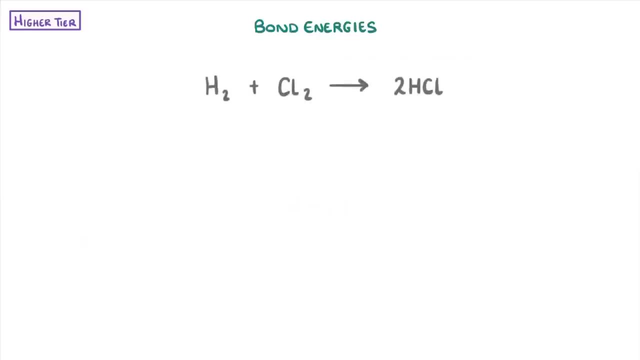 chloride bonds, it would release 431 kJ of energy to the surroundings. So if we took a simple reaction like hydrogen plus chlorine goes to form two hydrogen chloride and we were to think about it in terms of molecules, then we can see that for the reaction. 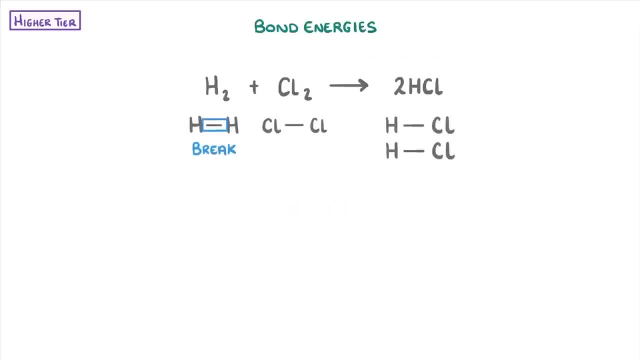 to work, we'd have to break this hydrogen-hydrogen bond. To determine if the overall reaction is exothermic or endothermic, though, we'd have to compare the total amount of energy required to break these bonds to the total amount of energy. 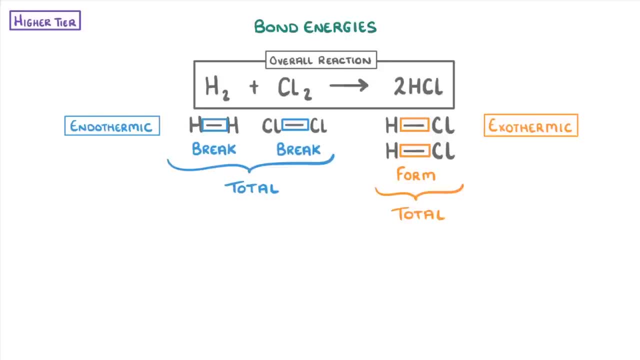 released when these bonds form. In an exam you'll normally be given a list or a table with all of the bond energy values that you'll need To work out the overall energy change. we just do the energy required to break bonds, minus the energy released by forming bonds, which in our case would be 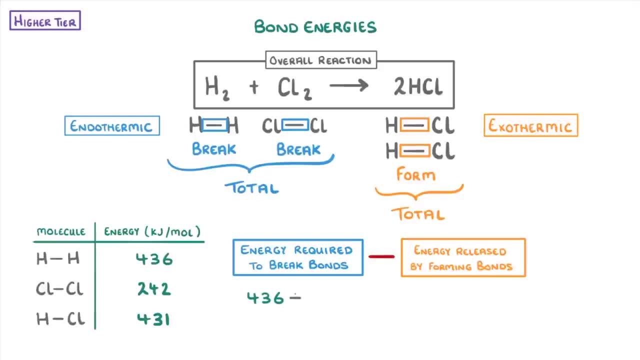 436 kJ for the hydrogen-hydrogen bond, plus 242 kJ for the chlorine-chlorine bond, minus 2 times 431 kJ for the hydrogen-hydrogen bond. So that's the total energy change we'd need to do. 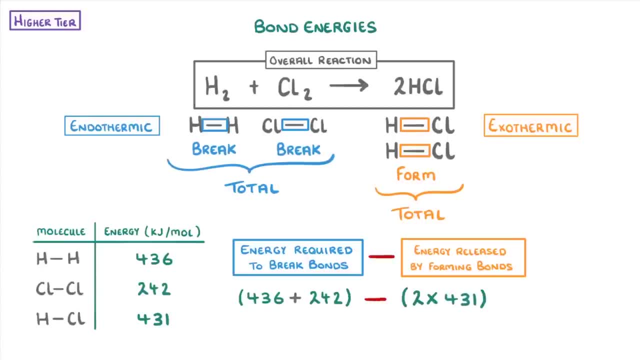 So if we were to take the energy required to break bonds minus the energy released by bonds within the two hydrogen chloride molecules, which simplifies to 678 minus 862, or negative 184 kilojoules per mole, And if you get a negative value like this, it means the reaction. 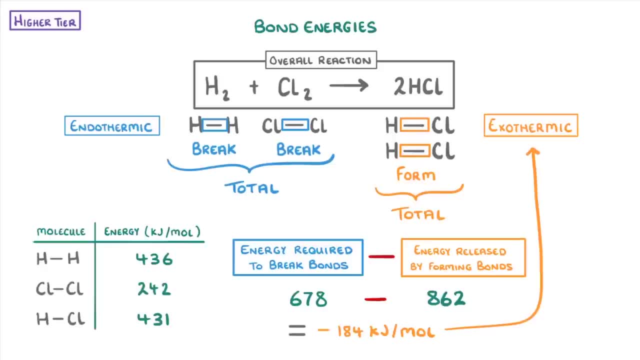 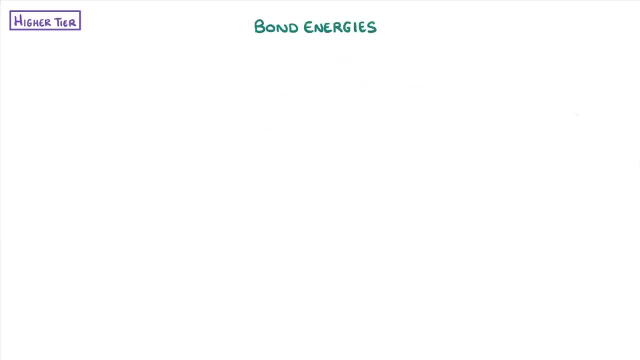 must be exothermic, as the chemicals are losing 184 kilojoules of energy to their surroundings. Before we finish, let's try one more example. Nitrogen and hydrogen react together in the following reaction. Calculate the overall energy change for this reaction. Now, although 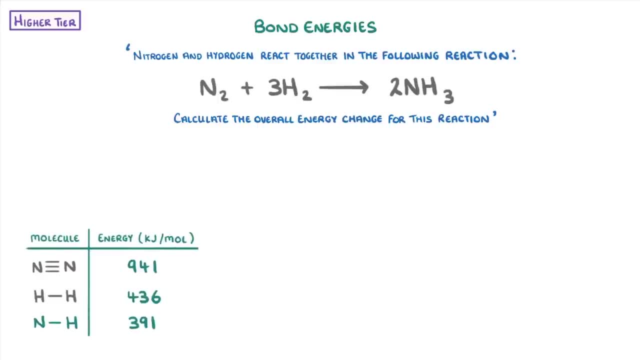 you don't have to. I think it's definitely easier if the first thing you do is draw out all the molecules using their displayed formula so that you can actually see the bonds. On the left, we can see that we'll need to break one nitrogen-nitrogen triple bond and